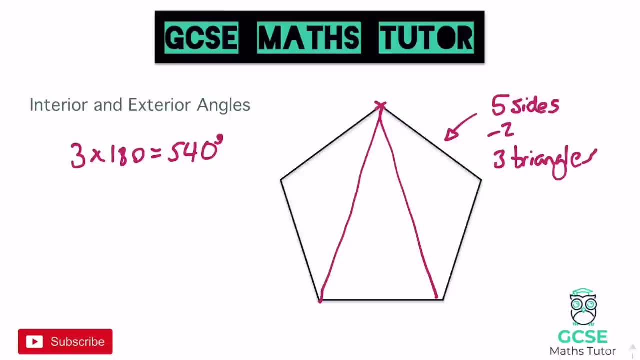 be applied to any polygon, and particularly with these regular polygons. If it's got 10 sides, you take away two and you do eight times 180.. If I've got 20 sides, you'd take away two, and that adds up to 4,, 5,, 6,, 7,, 8,, 9,, 10, 11.. That gives me a lot more room here. 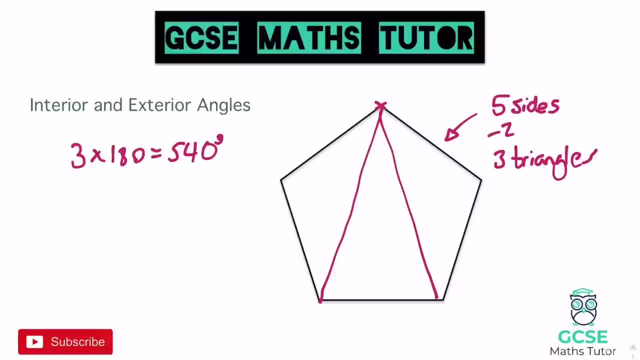 Okay, now if you were looking at an image and you're not a bigger polygon, you would think, and you do, 18 times 180. okay, so from there we can work out the size of one angle, because if there are five angles, we can divide that by five, and 540 divided by five, which can use a bit of a stop for. 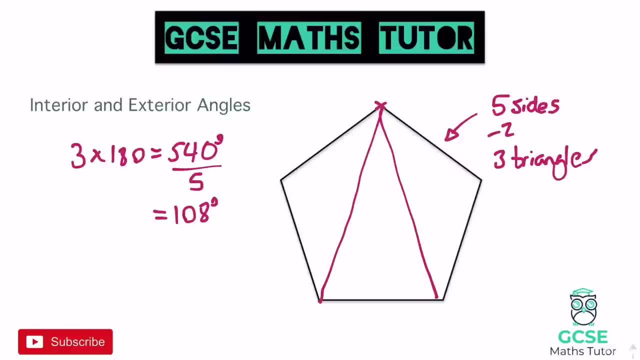 gives you an angle of 108 degrees, okay. so that's a good method there for finding the interior angle, and there's something else that we can have a look at as well. let's have a look and you can decide which one you prefer from here. so when you're looking at the exterior angle, i'm going 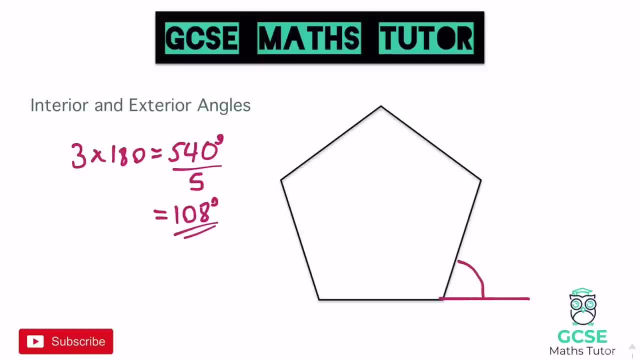 if i draw a straight line from the base here, the exterior angle here is what makes a straight line with the interior angle, bearing in mind. we already know the interior angle here is 108. we've just worked it out. okay, now there's something else that you can do to work out the interior angle. we know. 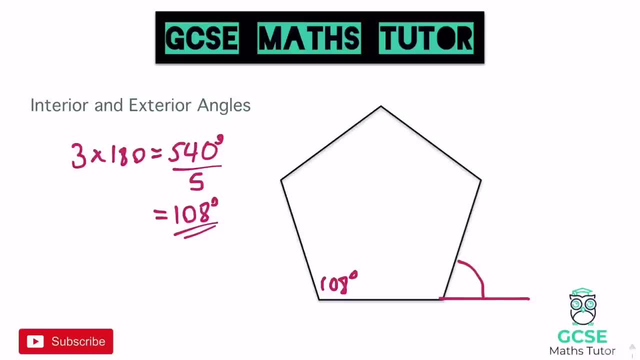 this is a straight line down here. now, the reason we look at this as the exterior angle is because if you look at all of the exterior angles, if i was to move around it in an anti-clockwise direction and kept drawing these little straight lines, all of these exterior angles here form a full turn. 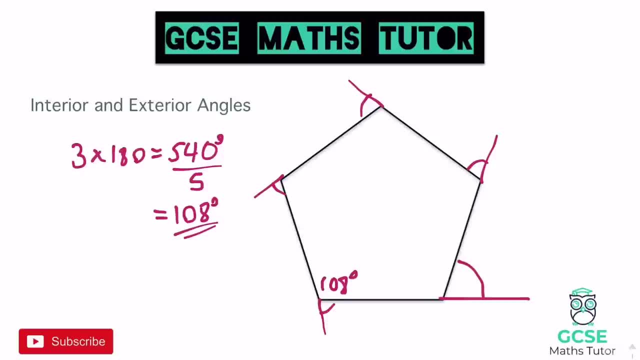 around the polygon. so a full, full turn there adds up to 360. so another way that i can work out the interior angle is to first think about the exterior angle. i can do 360 divided by the five angles there and it gives me an angle of 72 degrees. so if this one here is 72, we can do angles on a straight line to. 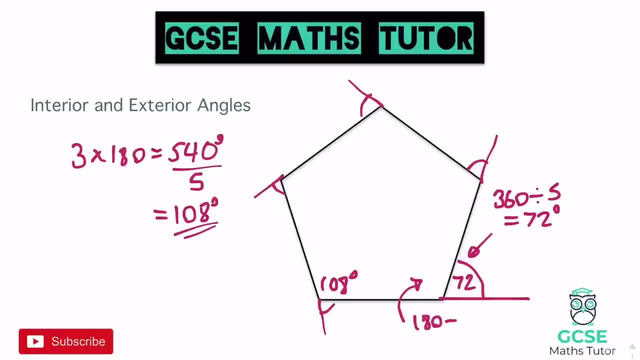 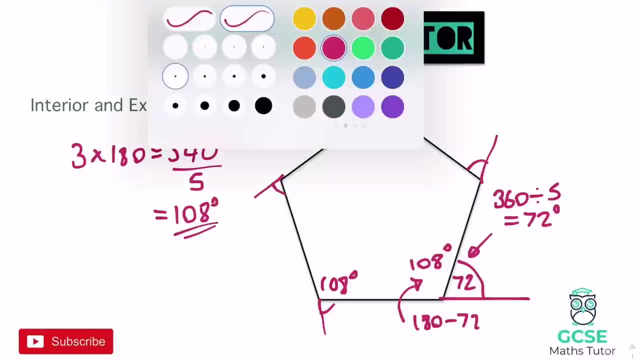 work out the interior angle and you can do 180, take away 72 and again. that's another way of finding out that it's 108 degrees. so there's two different ways there, two things that you need to know. so there's a straight line and a angle. so if you're looking at the interior angle, you can. 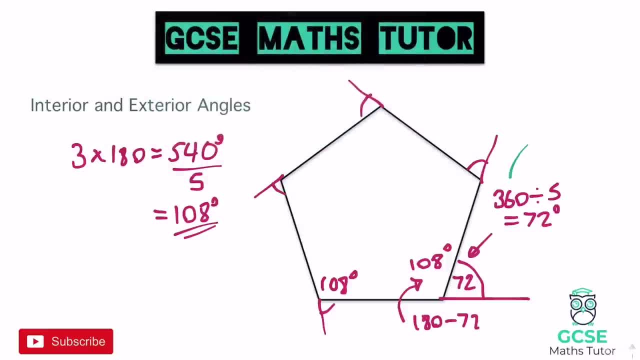 do a straight line and you can do any angle you want, but if you're only looking at your picture, you can do a straight line. so you need to know how to work out the interior angle and you need to know that the exterior angles add up to 360.. okay, so the sum of exterior angles. 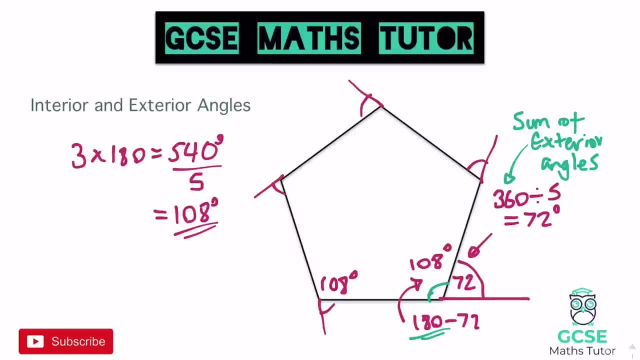 there we go, equals 360, and that allows you to find the exterior angle quite easily. and it's also- it's something that you need to know here- that the interior angle on the exterior angle add up to 180.. okay, so we're going to look at applying that. we've just got to remember, to find the interior angle, just take away 2 from the amount of angle you're going to need to use if you're going to use it as an example. 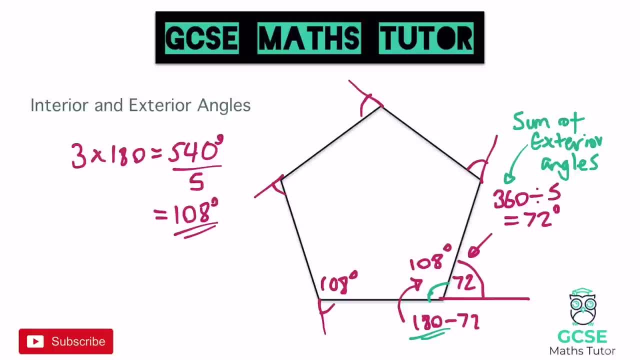 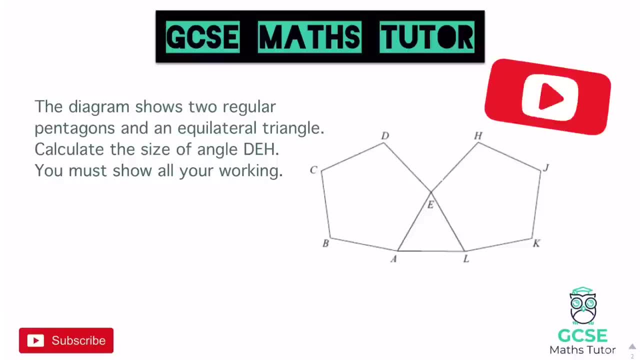 side, times it by 180 and divide it by however many angles are within that shape. so let's have a look at a little question on this. okay, so this question says there's two regular pentagons and an equal actual triangle, okay, and it says: calculate the size of angle d e h, which is this angle? here let's. 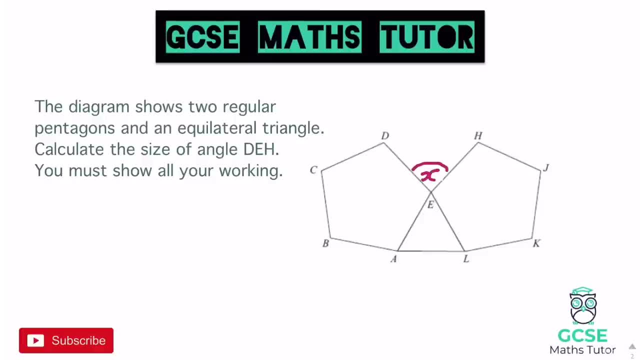 stick a little x in there and you must show all you're working. and this is really important on this type of question. you must show all you're working and you've got to show how you go about getting the interior angles there. so obviously we've just done a pentagon, so we know it's 108. 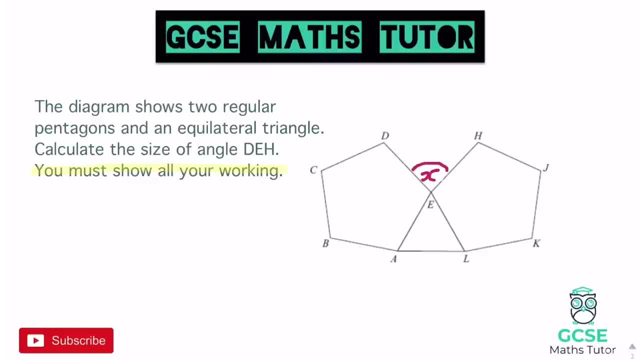 but just writing 108 in there wouldn't be showing my working. so whichever method you decide to do, i'd have to do show my work in there. so i'd do 5 minus 2, which equals 3, 3 times 180, which gets me 540. you might have to do some written methods here and then divide that by 5. 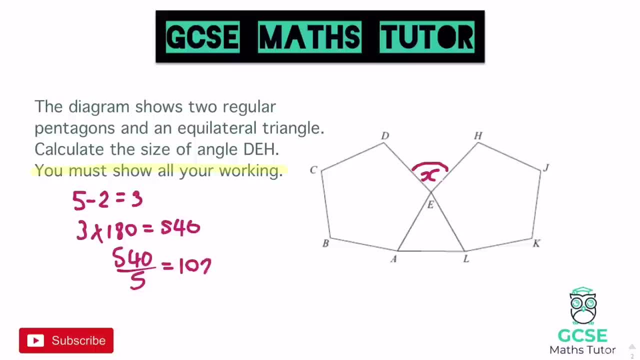 so 540 over 5 gives me the angle of 108 and that is me showing my work in there, how i get the angle inside the pentagon, so we can put that in 108 and i can put in 108 here now the reason i've gone for. 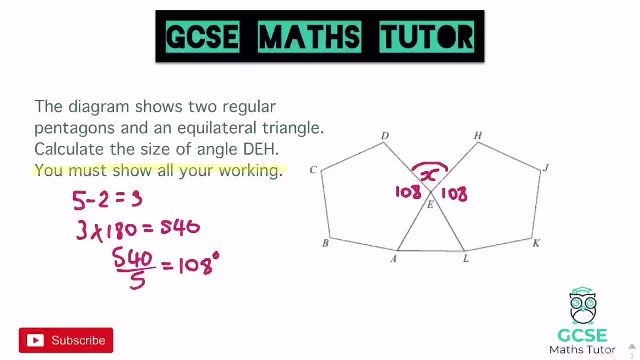 this question is because i've got a lot of angles and i've got a lot of angles and i've got a lot of corner here is because they're all slotted together. we're looking at angles around the point here and we know the total of all these angles is 360 degrees. so 360 degrees around a. 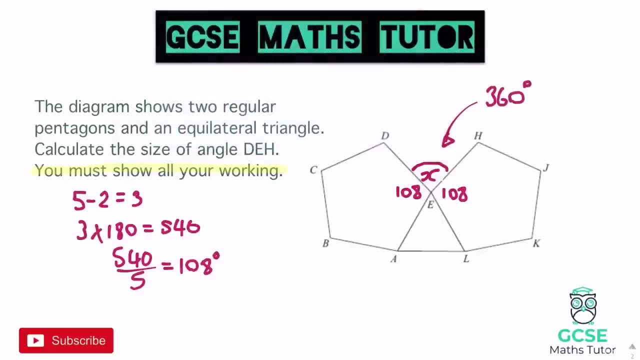 point. the final angle here that we have to find is the one inside the equilateral triangle. now, we don't for an equilateral triangle and a square. we don't actually have to show our working for that. it's presumed that we should know those. and inside an equilateral triangle the angle is 60. 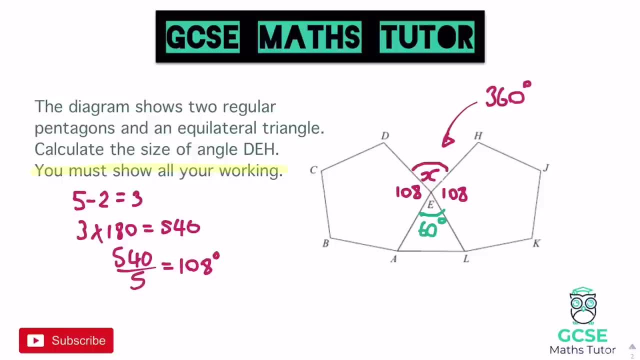 there we go. so if these have all got to add up to 360, all we've got to do is add these all up, so 108 plus 108 plus 60, and that gets us 672, so 276 degrees, and we just need to take that away. 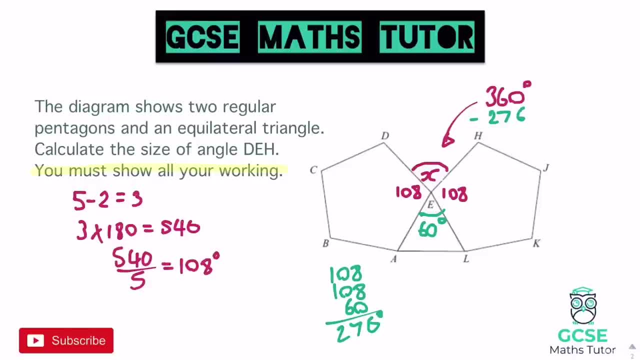 from our 360 up there. so take that away, take away 276 and that leaves us with 60, 70, 84 degrees. there we go. so our missing angle there is 84 degrees. okay, showing all our working in stages as we go. so first things first, we worked out the pentagon. 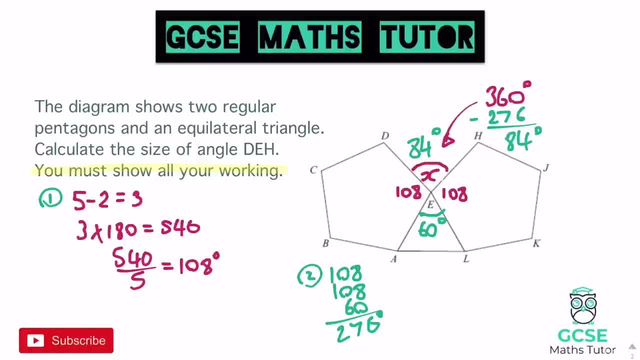 then we added up all our angles and then we took it away from 360 to find our missing angle there. so nothing too horrible in these questions again. you've just got to make sure with this type of question you label everything all over the diagram, write the angles in everywhere and just make sure it's all. 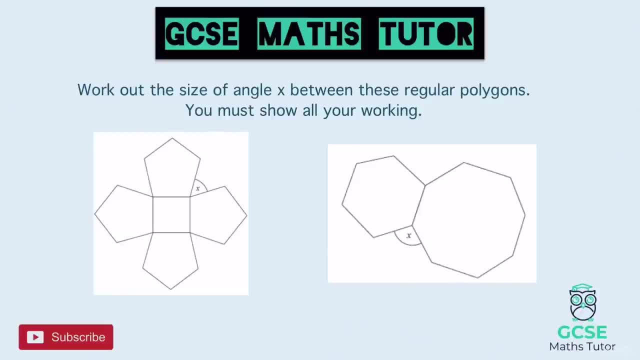 really nice and clear. so here's some for you to have a go at. so have a go at these two. find the size of angle x in between these regular polygons. pause the video there. we'll get the answer in a sec. okay, so the first one here. now we're going to show all more working for this one, obviously. 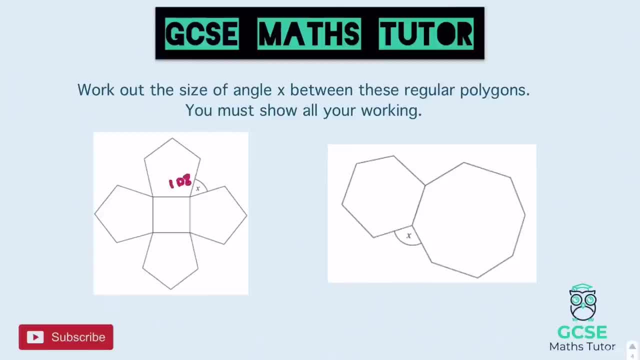 we've just done the pentagon, so you would need to show all the working for this one. we're going to show you working, but we know that this angle here is 108, this angle here is 108 and this angle in this square is 90. okay, and then, finishing that off, obviously these have all got. 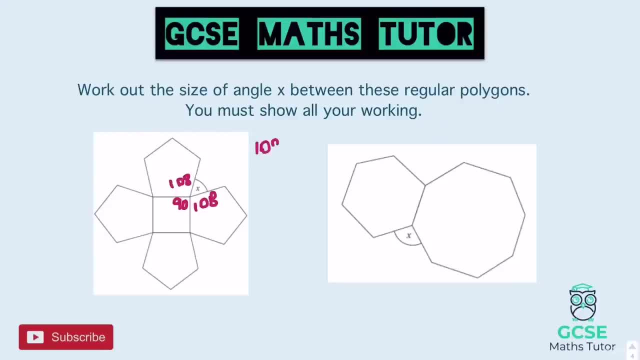 up to 360 around the point. so if we add those up we've got a 108, 108 and 90 and that adds up to 603, 306 degrees, and then take that away from 360. so 360, take away 306 and that leaves us with 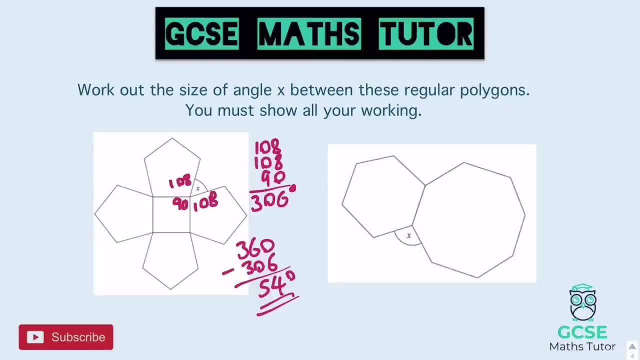 54 degrees as the angle x there, so let's just label that on. do it in a different color. 54 degrees is the answer to our first one. obviously it's just showing you're working for this 108 here. on to the next one, we've got a hexagon so we could work out the size of this angle here. 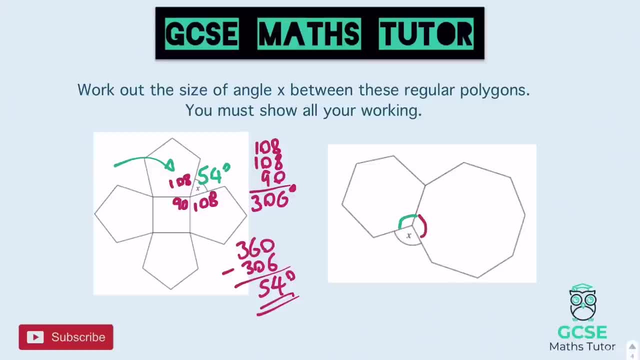 and we've also got an octagon there with eight sides and then that'll be this angle here. so they're working out for the octagon. let's work this one out. so there's eight sides, so eight take away. two is six times that by 180, so six times 180. 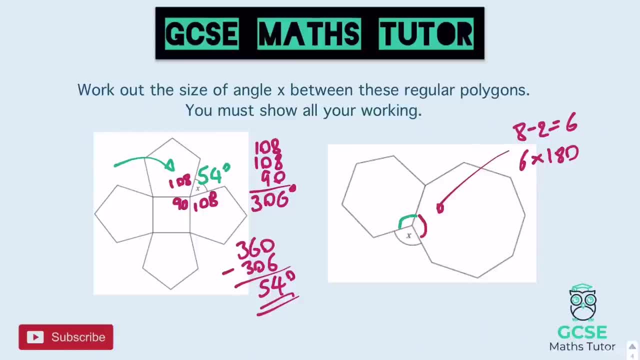 and six times 180. obviously, if you have a calculator, that's nice and easy. if not, you are going to have to just do some written methods for that. make sure you get it right. but it's 1080. lovely, it's got eight sides, so divide it by eight and we'll get the answer 135. 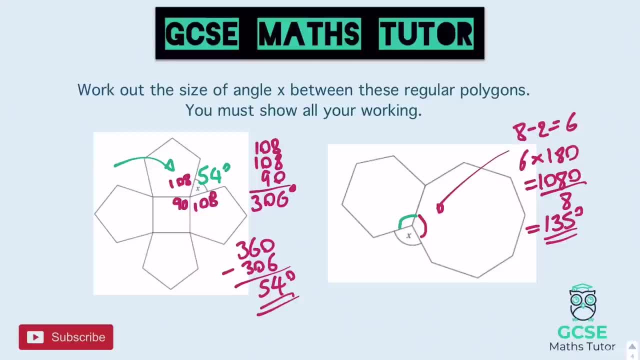 degrees. okay, so there is the interior angle in an octagon, so there we go, 135. the next one we have to work out is the hexagon. so this angle here. so it's got six sides. so six, take away two, which is times up by 180, gets you 720, and then it's got six sides. so divide that by six and we get 120 degrees. 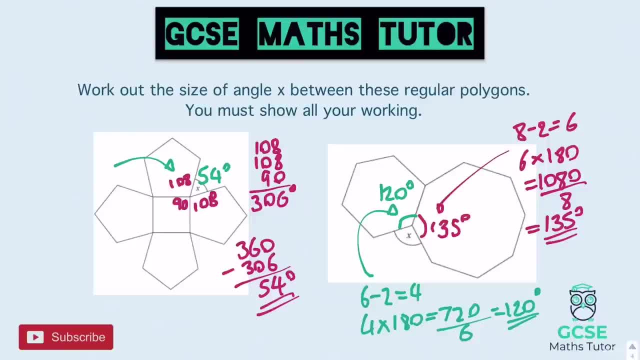 for inside the hexagon. so 120, and then, finishing this off, we just need to find the size of the missing angle there. so add these both together, so 120 plus 135 leaves us with 255 degrees, and then take that away from 360 leaves us with a missing angle here. let's do it over here, just to. 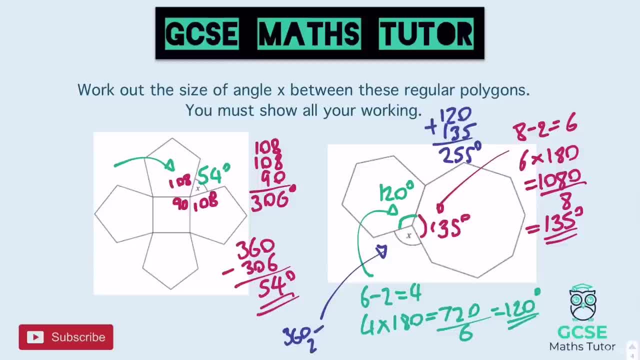 show our working out: 360 take away 255 leaves us with 105 degrees for that angle. there, all right, and there we go, and that's how to work out some of these problems when you've got polygons fixed around a point. so i'll look at one more before we finish, okay, so here's quite a different. 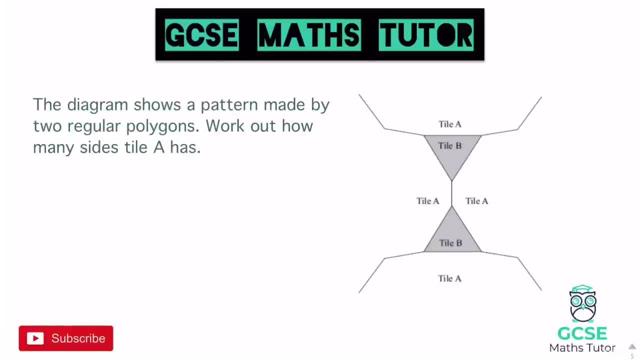 question. it says the diagram shows a pattern made by two regular polygons. work out how many sides tile a has. and what's not very nice about this one is it doesn't show you, um, all of the sides here. obviously. that's why it's asking us how many sides it has. it just shows us part of tile a and 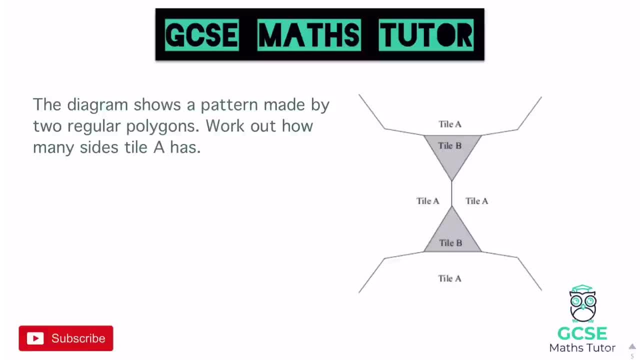 equal actual triangle there. so have a go at this one, see if you can work it out. i'm going to go over the answer, but see what you get, see if you can figure out how to apply some of the methods we went over in that first um, that first slide there, and see if you can get the answer. so pause. 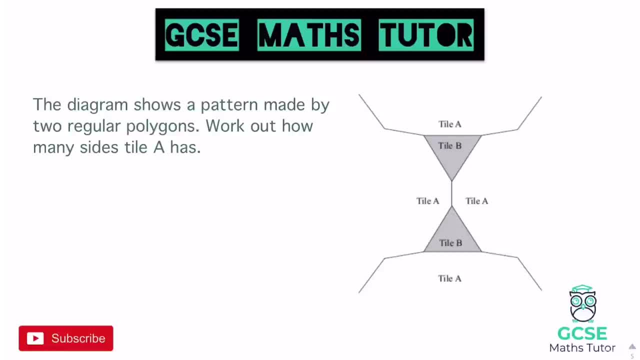 the video. have a go and we'll go over the answer in a sec, okay, so looking at this question then now, first things first, let's have a look at the angles around this point right here now. we know, in the equilateral triangle that's an angle of 60 degrees, and if tile a is the same on both sides, 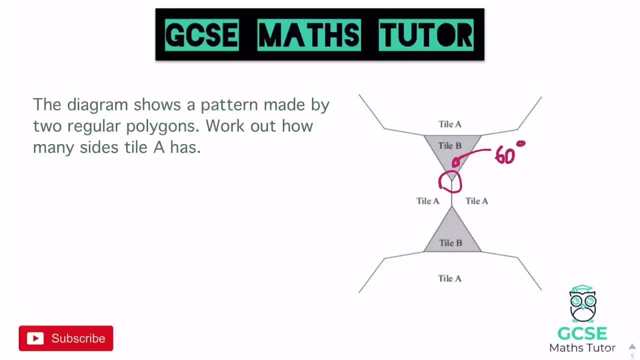 then, um, what we can do is take that 60 away from 360 and split it in half. so if we do that, so 360, take away the 60 degrees in the triangle, leaves us with 300, and if we divide that by 2, we've got 150 degrees in each of these tile. 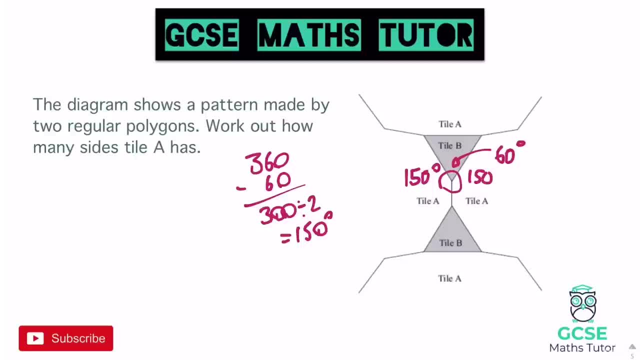 a's here. so 150 degrees and 150 degrees. so what the question is now asking us is what polygon, or how many sides, does the polygon, have to have to have that interior angle of 150 degrees when it's a regular polygon? so two different ways we could do this now. we could just 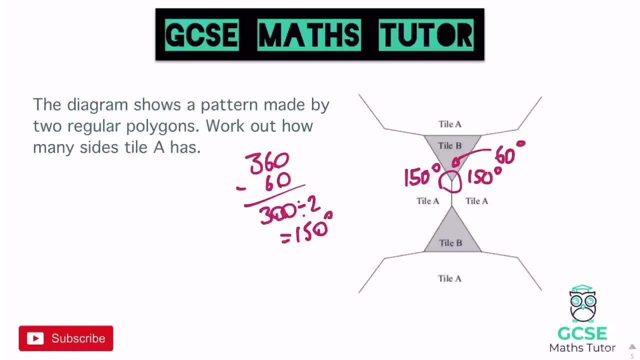 guess i could just say: okay, let's just guess 14 sides, and then, if it is 14 sides, i'll take away 2 times 180, divide by 14 and see if it matches, and if it's too high i'll go, i'll go lower, and 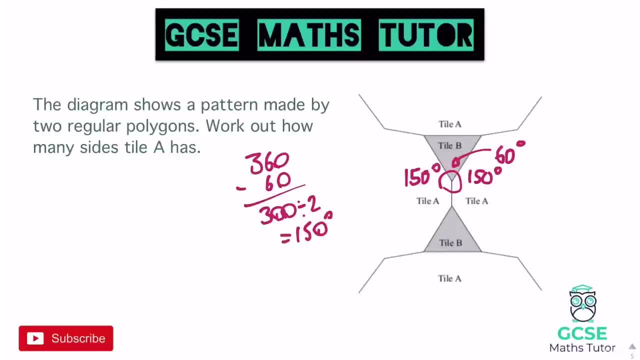 if it's too low, i'll just go higher with my sides, okay, but we can take a little bit of a an easier approach here now. if you remember, on that first one, when we looked at the polygon, if it had an interior angle of 150 we could have a look at what the exterior angle is. and because it's on 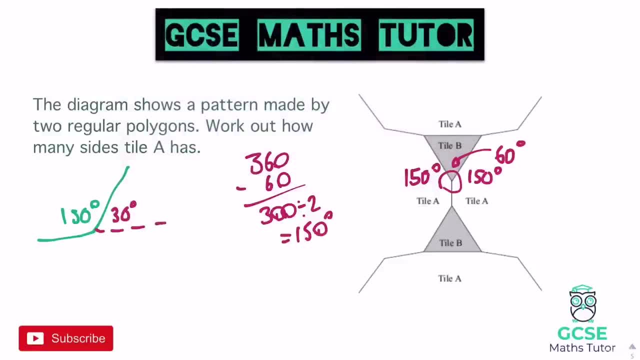 a straight line, the exterior angle would be 30 degrees. so if you think about this, if you remember that all the exterior angles add up to 360, well, if one of them is 30, obviously 150 and 30 make 180, then i could just say, all right. well, if 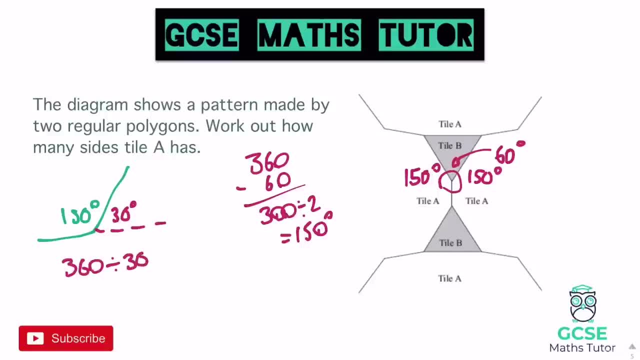 i do my 360 and i divide it by the exterior angle there, which is 30. that gives me a total of 12.. there we go, and that tells me that there must be 12 angles around the polygon, because obviously that 30 fits in 12 times. so there we go, working that out. then we've got 12 sides. 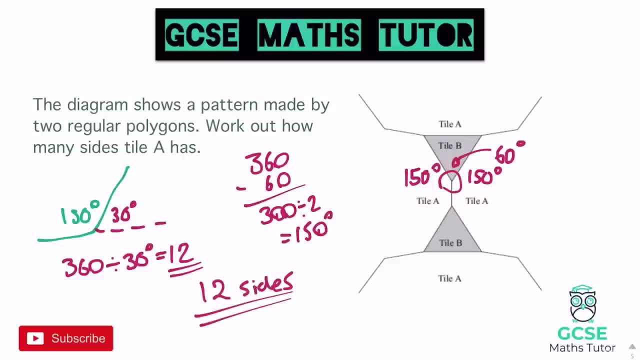 as our final answer. and again, you can check that. if i was to do um 12, take away with 2- that'd be 10 times 180- and then divide it by 12 and you get the answer 150. so you can always check that out. 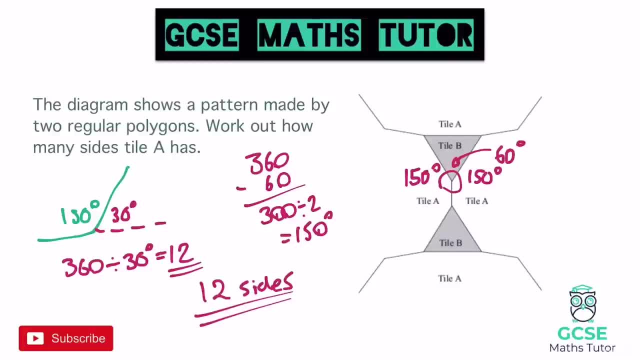 but there you go. that is the end of polygons there. i will do some harder questions on polygons. these ones are quite nice, but i will have a look at doing some harder ones in another video. but just a little quick one on polygon. saw you there, so that's the end of the video, if it was. 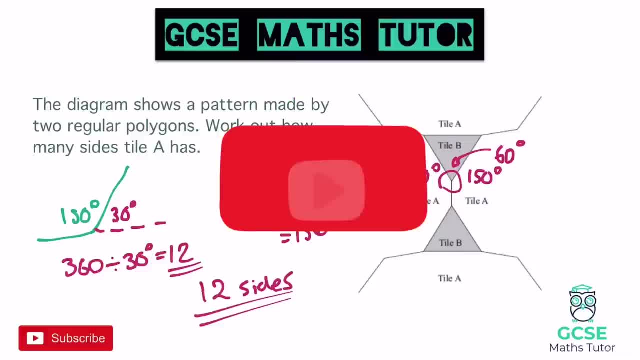 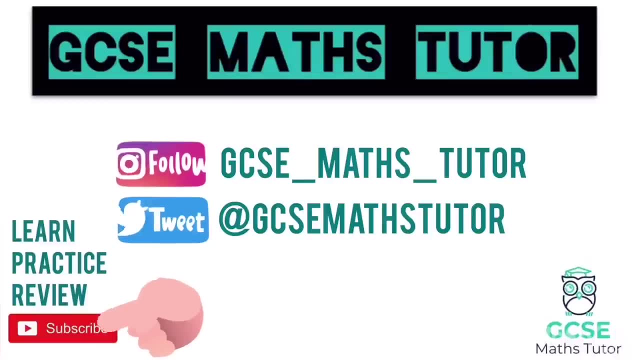 helpful. it was useful. please like, please comment, please subscribe and i'll see you for the next one and i'll see you in the next one.